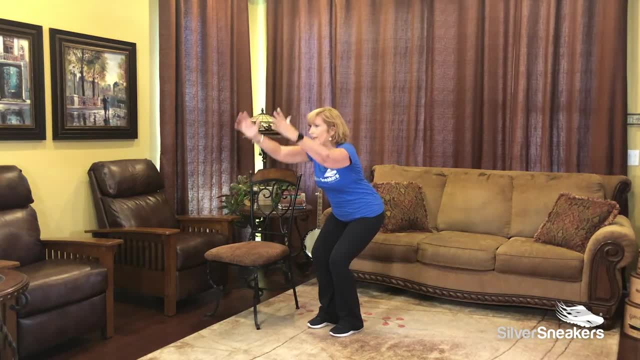 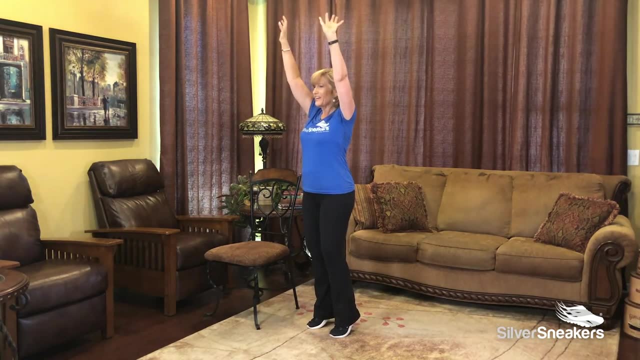 chair, Sinking the hips Back so your knees are over your feet. Exhale, stand up and then inhale. reach up high, Hold All right, shift the weight side to side. It's okay to wobble a little. Your body's adapting and 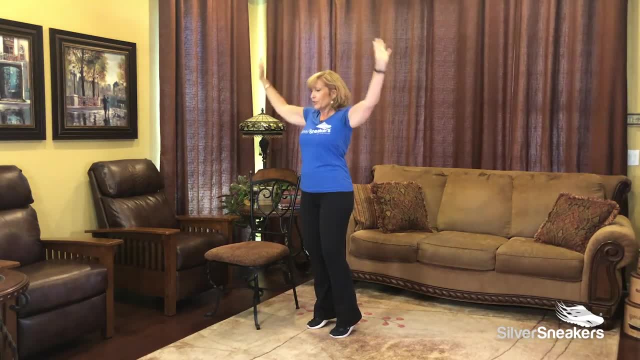 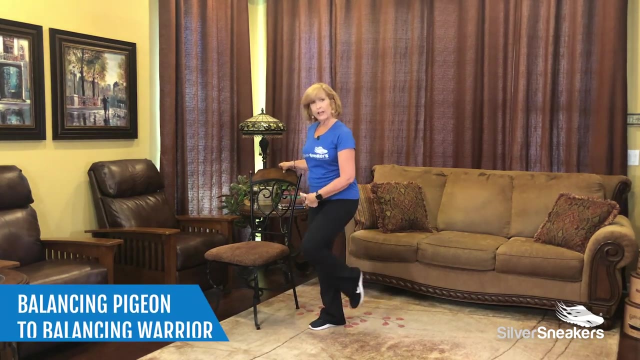 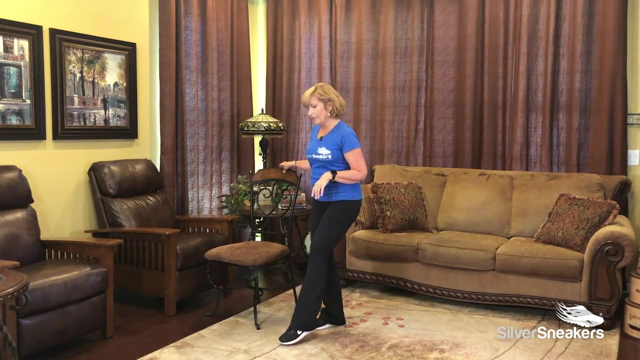 trying to stay stable. You're working. Then bring the arms back down, All right, as we move towards a balancing pigeon. we'll start with option number one. Touch the right toe forward and then touch it back. Your standing leg remains a little bit bent as a shock absorber. Now, if you need more challenge, 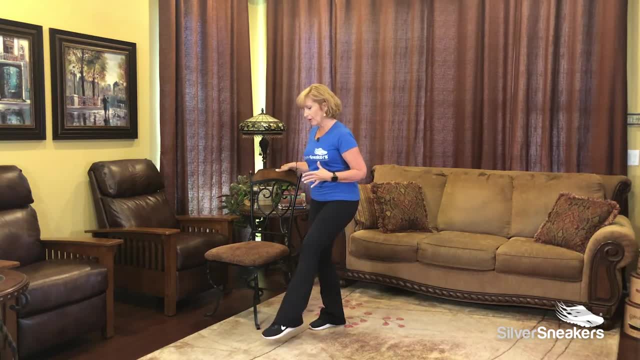 you can take your hand away from your countertop or chair, or you can cross over to the opposite side instead of straight ahead, and then slide back and lift the toe off the floor, reaching through the heel- So opposite side, And then reach or slide back, reaching through the heel. Your hands can come next to your hips here. 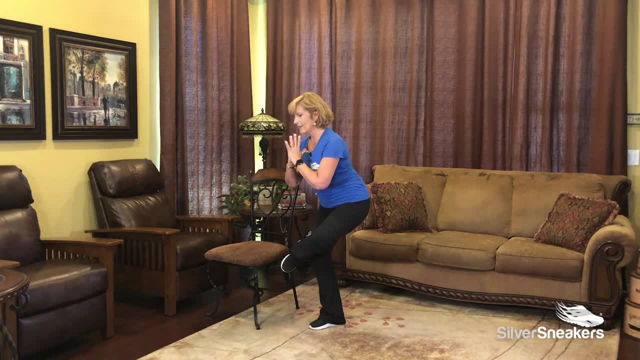 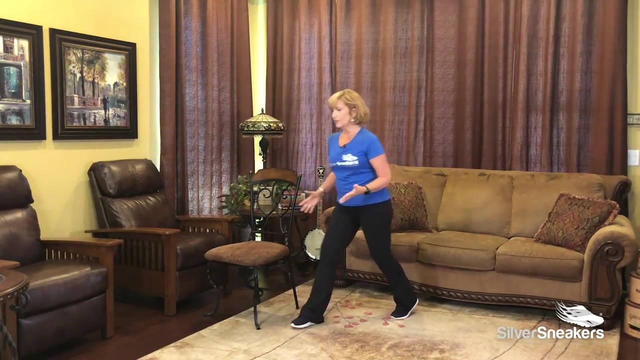 or for the third intensity option, sit down like you're in a chair, sink your hips back, hands at heart center, and then reach back, extending through the heel, challenging yourself with your balance. and then let's step the right toe back into a split stance, but really more of a lunge: Hips tuck under hands to heart center sink. 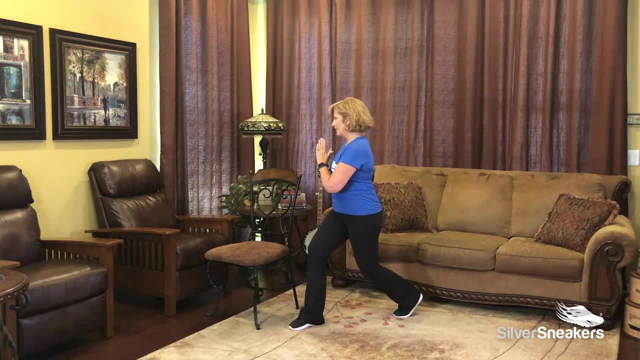 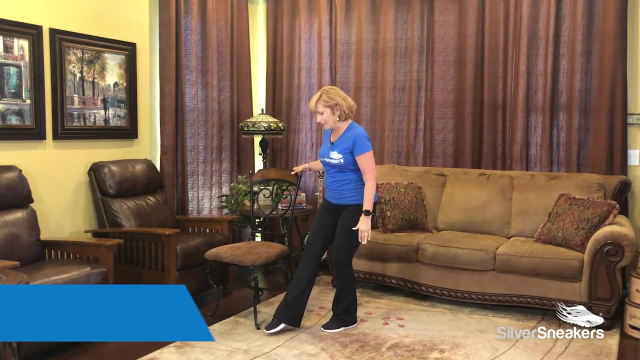 remember your front knee is right over your ankle and then we'll twist to the left and come to center. so keep looking right over your hands to challenge your balance more Great. let's step to center and do the left side, starting with that balancing pigeon, touching. 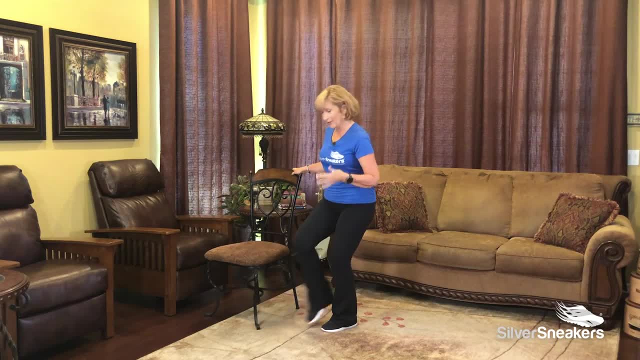 forward and back. is that the option for you today? or we'll cross center and then slide a few inches above the floor- You're using your chair as much or as little as you'd like- and then sink down into more of a pull, a full balancing pigeon.